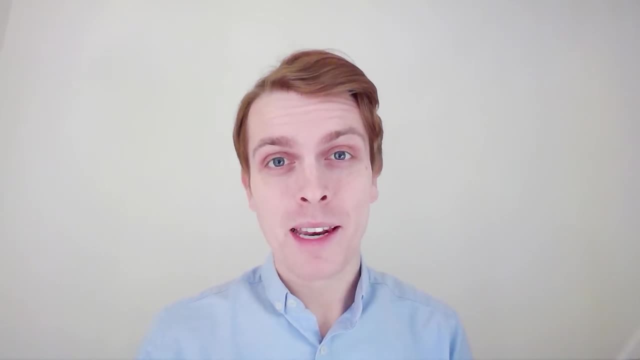 protection law is and why it's worth your while to spend just a few moments thinking about it. Do data protection laws apply to most small organisations? Whether you have staff or trade by yourself, you're likely to collect the personal data of the people that you come into contact with, whether that be customers, suppliers or even 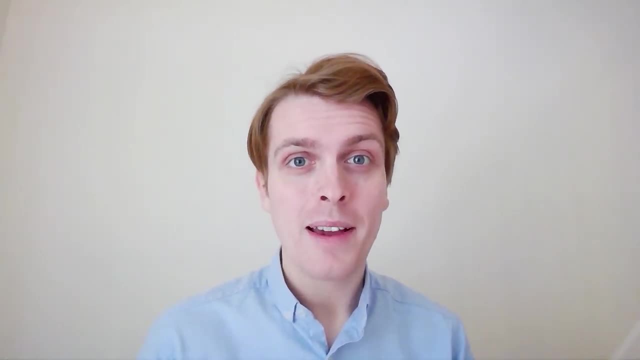 the people that you employ. For example, you might collect a person's name and address to send out a product to them, or their email to send out a service update or a newsletter. Regardless of the type of personal data that you collect, it's important you use it reasonably. 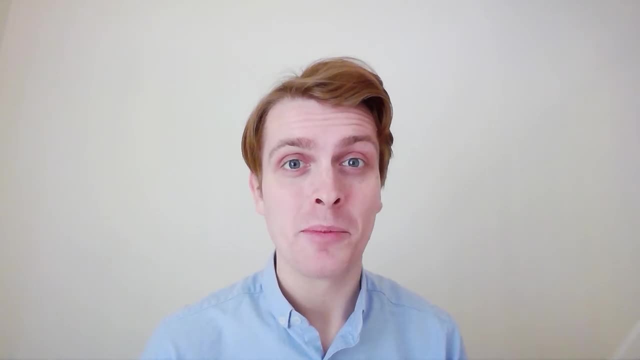 and protect it, as this is what ultimately underpins data protection law. The reasons for this should hopefully be quite apparent. If personal data falls into the wrong hands, then people could be harmed. This could be as a result of identity theft, discrimination or even physical harm. 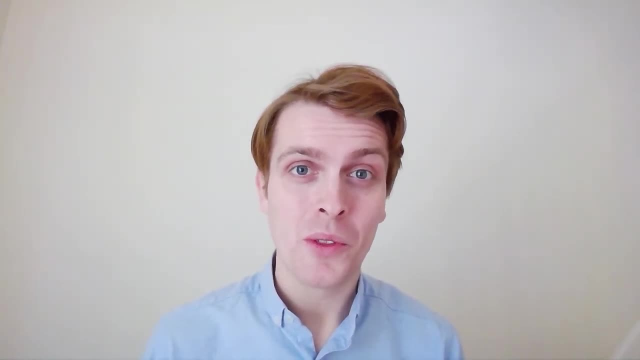 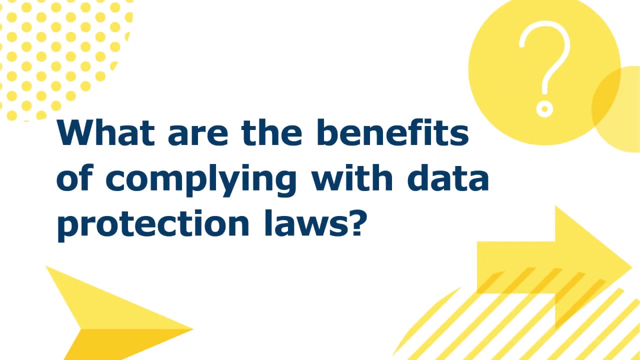 So data protection law explains what should be done to ensure that everybody's personal data is used both properly and fairly. Generally speaking, it applies to all types of workplaces, business ventures, societies, groups and clubs. What are the benefits of complying with data protection laws? 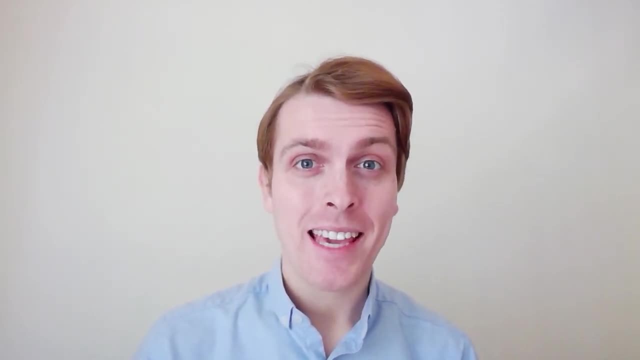 So, firstly, it helps to build trust, as keeping people's personal data secure is key to getting them to trust the service you offer and, more broadly, your business as a whole. This should help to build up both your reputation and your brand. Alongside this, it also makes 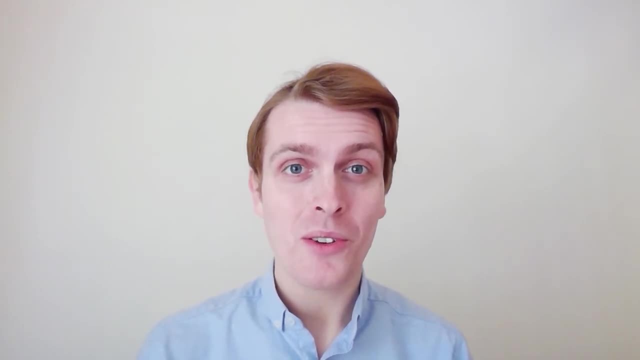 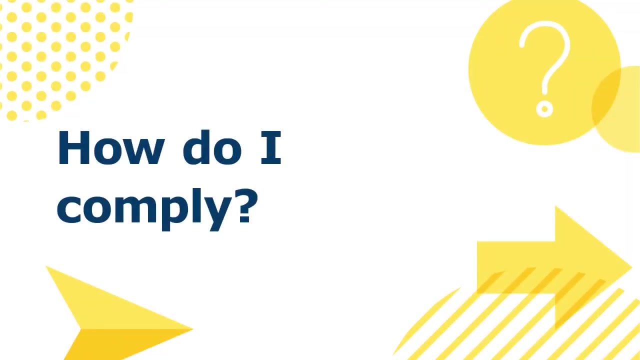 good economic sense, As adhering to data protection law should end up saving you both time and money. It should help to make sure that you don't incur any unnecessary costs on storage, as well as allowing you to deal with any requests you might receive in a timely manner. 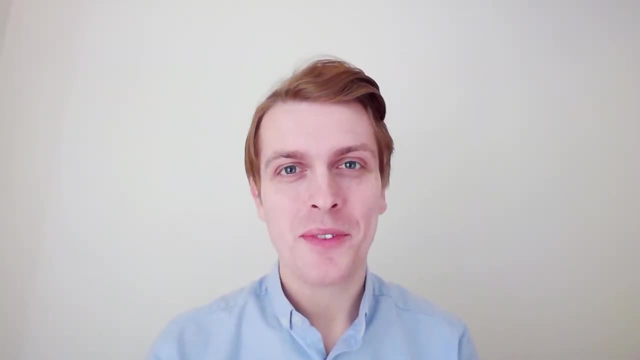 How do I comply? There's no one-size-fits-all approach to data protection law. Your business is unique, and that's what makes it great, And your approach to data protection law will be unique as well. It's going to end up being much easier than you think, but it's also going to be a lot. 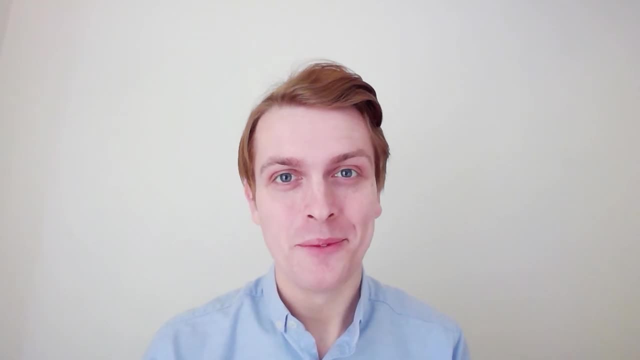 easier than you think And we're here to help you make any changes you might need to. As a great place to start, it's worth checking out the resources on our Data Protection Hub for Small Organisations, which contains loads of tools, top tips and bite-sized guidance.